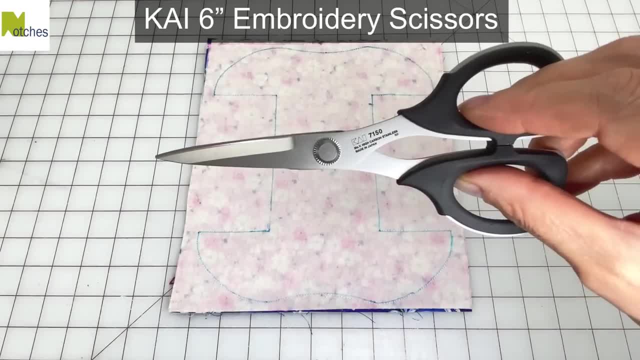 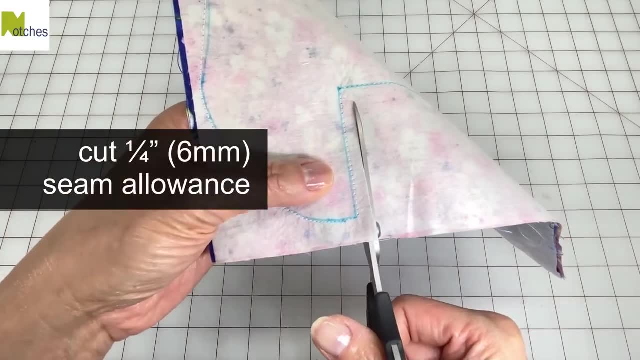 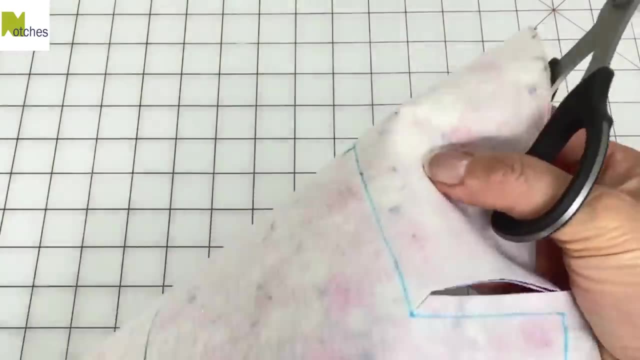 I'm using my Kai 6 inch embroidery scissors for the trimming Cut all around, leaving a quarter inch seam allowance At the inner corners, cut right into the point, making sure not to cut the stitching. If you're finding this video helpful, make sure to like. 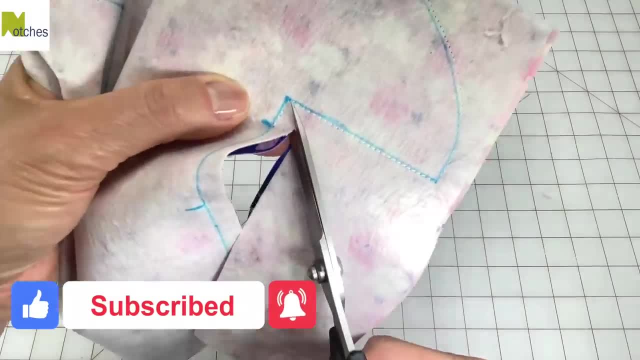 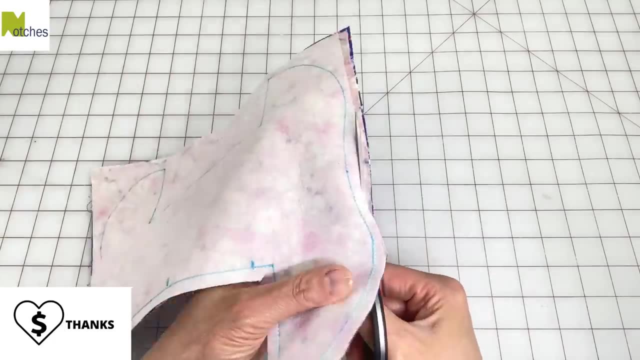 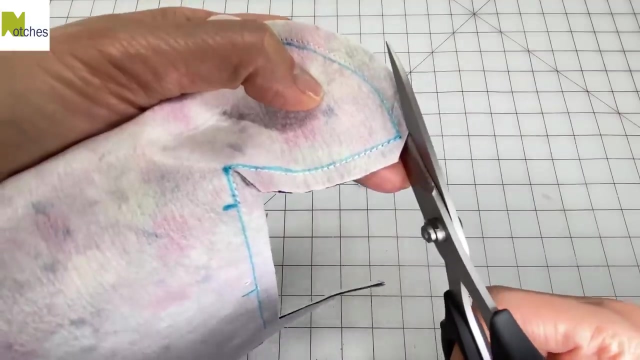 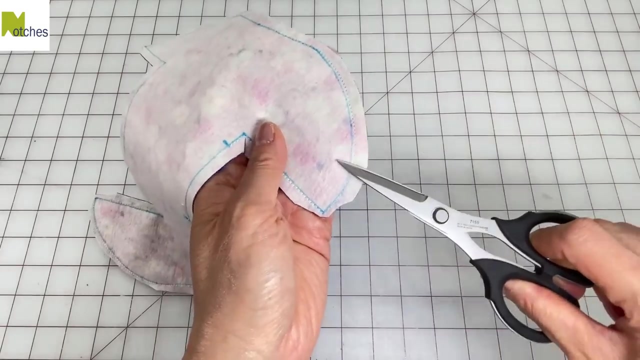 share, subscribe and turn on all notifications and also leave a comment below. At the outer corners, trim on an angle and then trim a little bit on each side again, making sure not to cut the stitching. For less bulk along the outer curves you can trim away half of the seam allowance down to 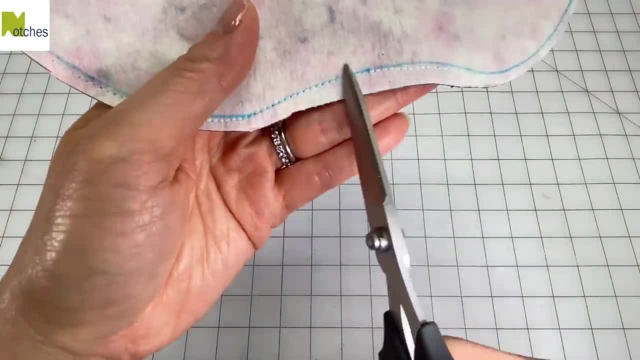 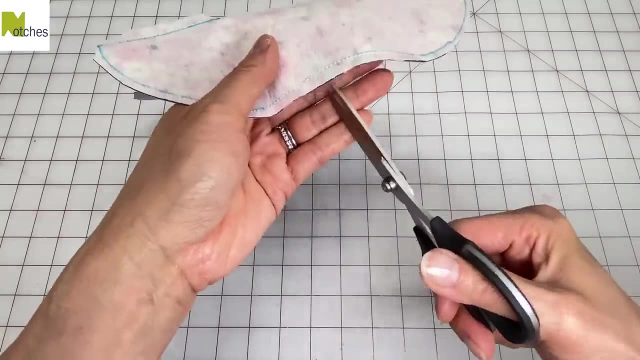 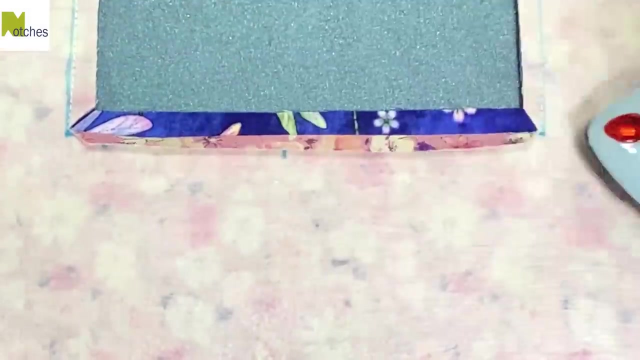 about an eighth of an inch Along the inner curve. cut notches into the seam about half an inch apart. Spread apart the seam where the opening is and press flat. Turn over and fold down the other side of the seam and press this flat as well. Then press open. 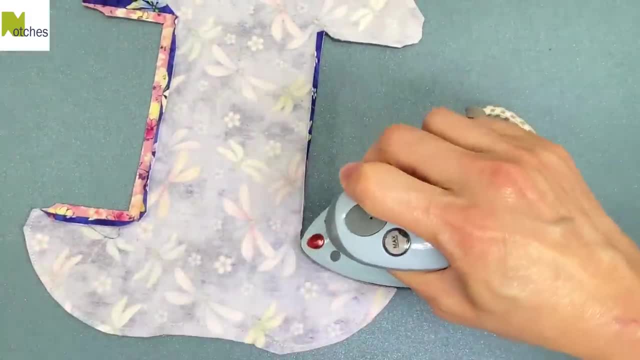 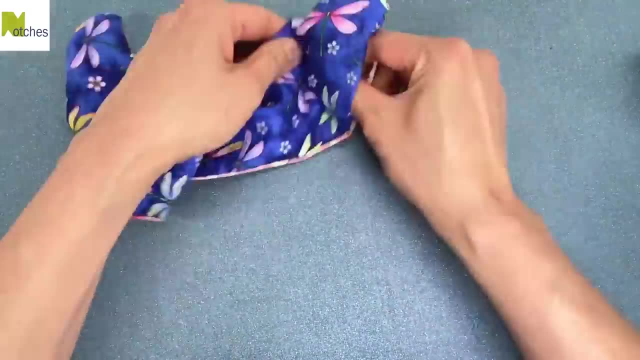 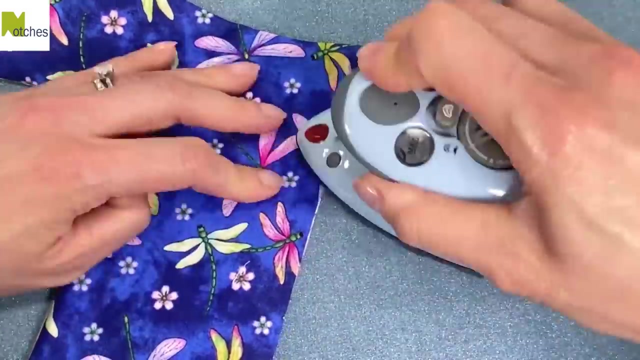 the rest of the straight seams. Carefully. turn it right side out and then use a knitting needle or a point turner to push out all the corners and the curves. Roll and adjust the seam so that they're right in the center and press all. 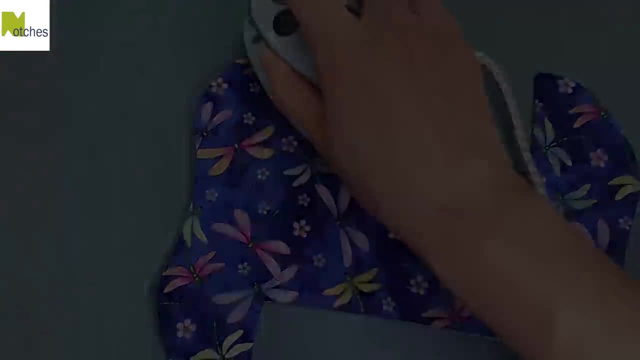 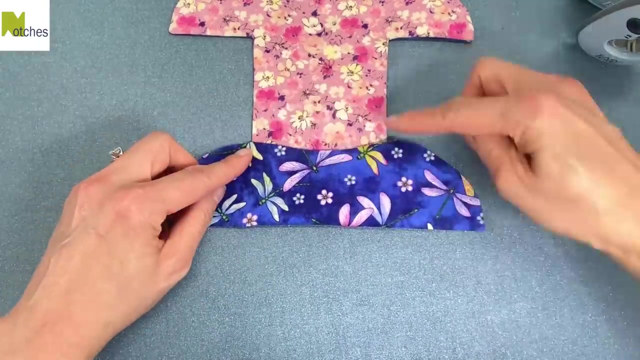 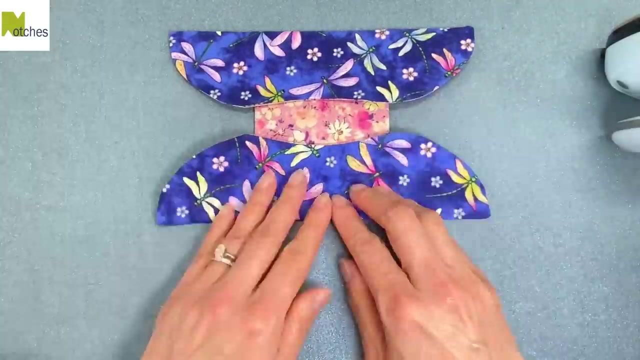 around With the lining side up. fold one end at the corners straight across- These peaks should be in line with the side edges- and then press across the fold. This edge should be nice and straight. Now repeat on the other side. Fold the. 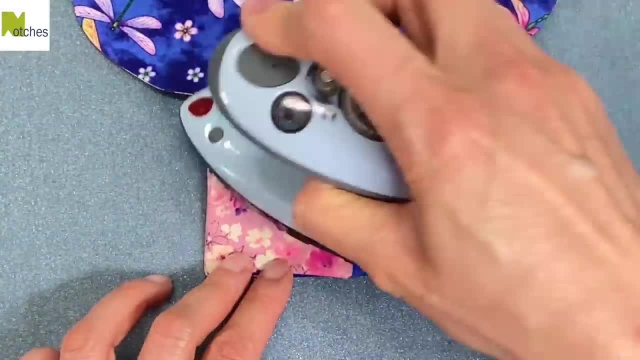 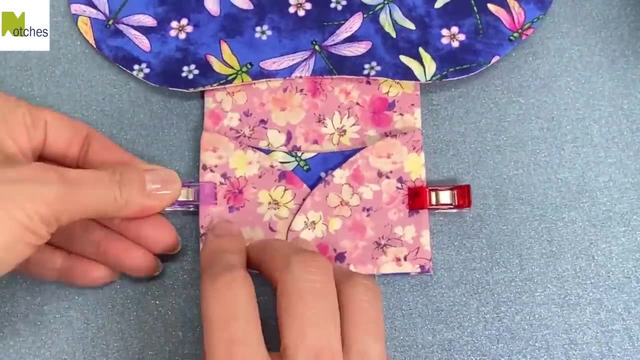 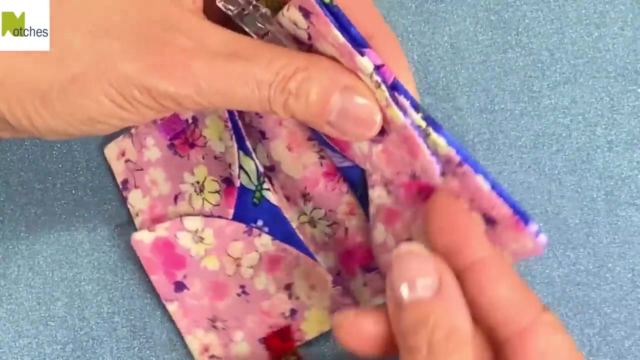 left side so that it's in line with both edges. Give it a press, fold the right side and press Clip in place and then repeat on the other side To find the center between the layers. fold this top corner back to match the bottom corner and then mark. 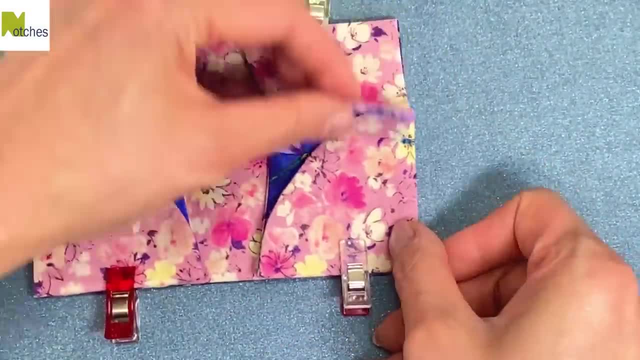 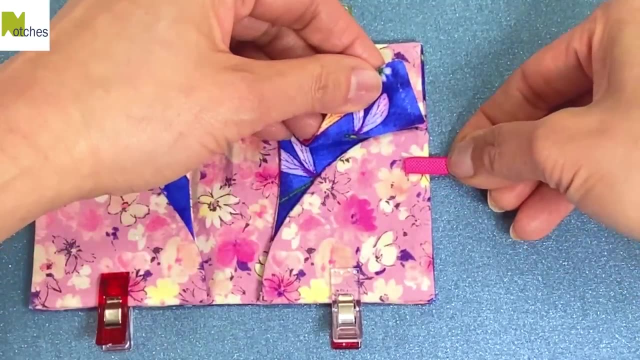 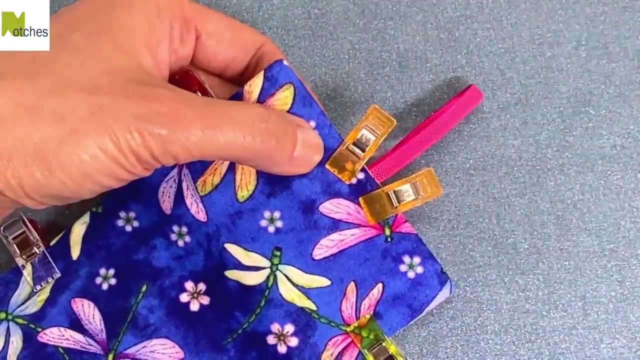 the bottom layer. Fold your elastic in half lengthwise, with right sides together. Place the ends on that center. mark between the top two layers about a quarter of an inch in from the center. Fold the top corner back to match the bottom edge. Turn over and clip in place on either side. Increase the stitch length to.